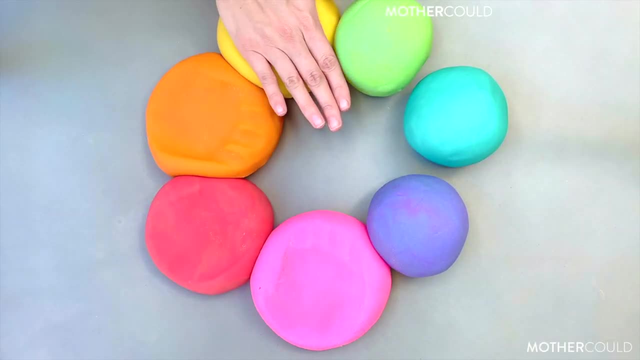 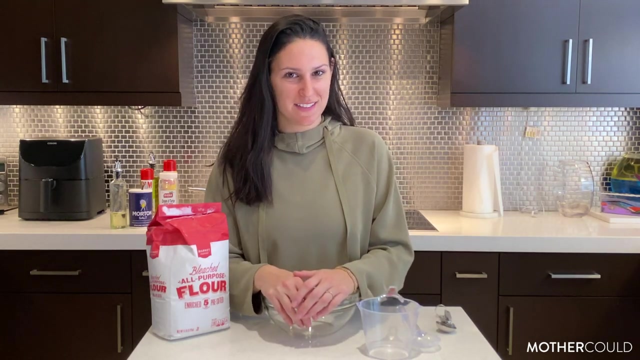 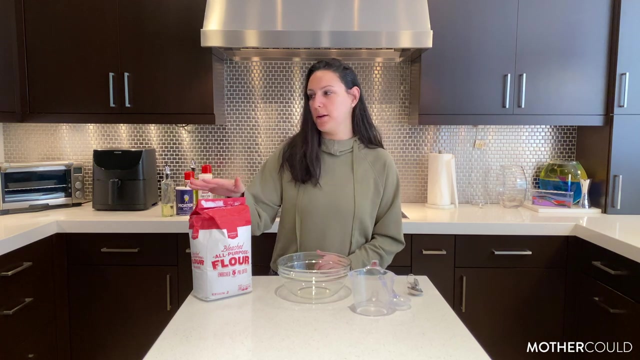 Let's make play-doh. Hey guys, today we are making my all-time favorite play-doh recipe. It comes together really fast, so let's get started. First things first, let's gather all our ingredients and have them around your bowl. So I have my flour here and the rest of my ingredients back here, as well as my water. 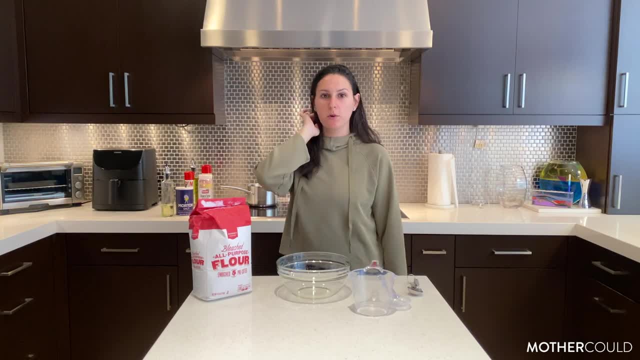 already in a pot, And the first thing I'm going to do is put the water to boil, because I want it to be ready by the time I need it in my bowl And, like I said, it comes together super fast. So now that the water is boiling, I'm going to take my measuring cup. 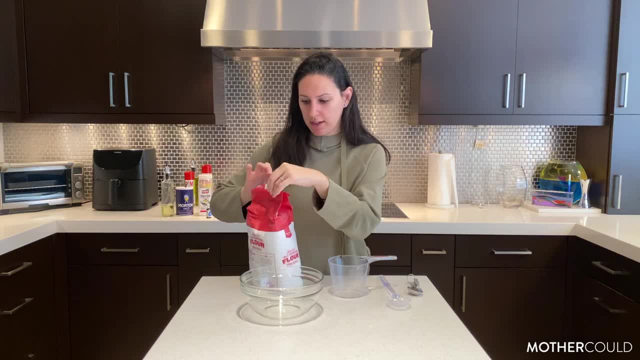 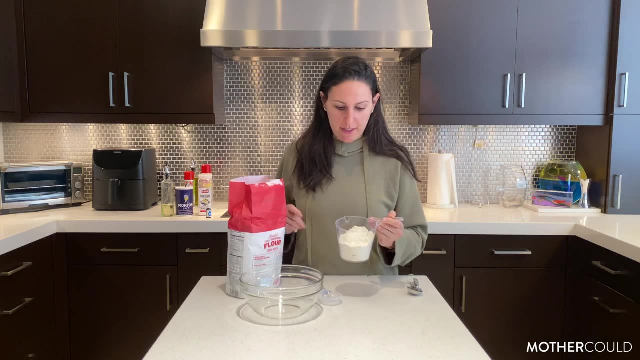 and I'm going to measure the flour because it's the first ingredient in our play-doh. The trick with this play-doh is to pat down the flour already in the cup, So we want it to be really compact to get an accurate measurement. 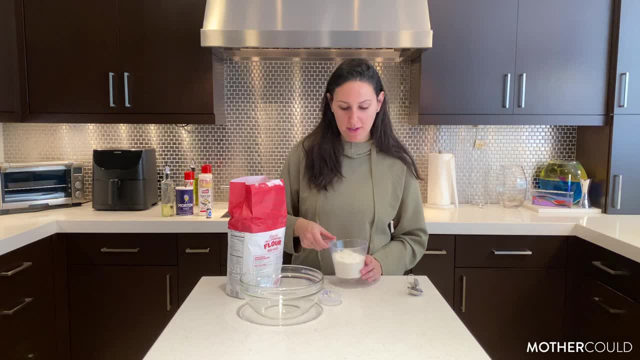 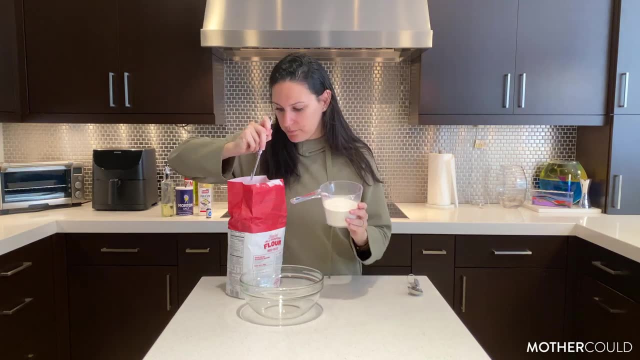 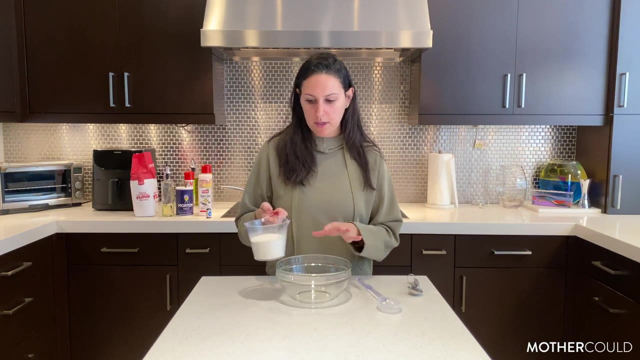 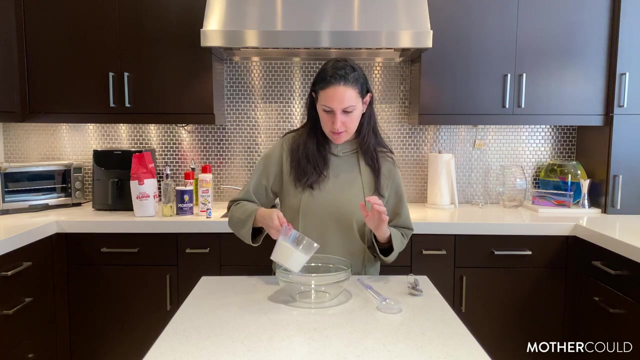 So I'm just going to bang it onto the table and compact the flour to make sure it's one full cup of flour. So I'm going to pour my flour into my bowl And the way you know that it compacted well is that it holds the cup shape. So I'm going to turn it. 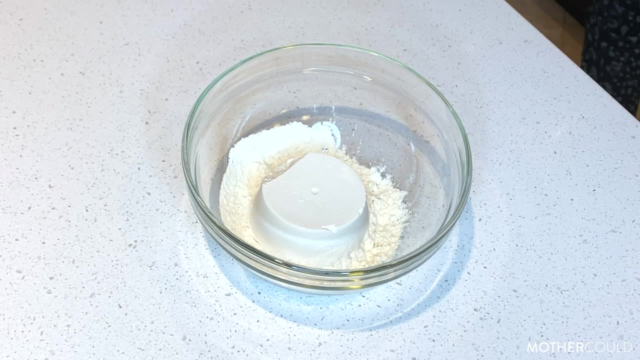 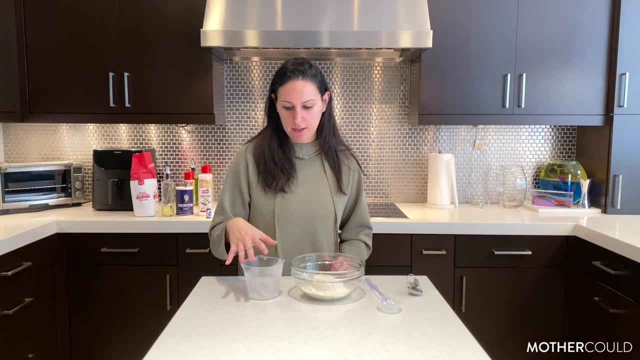 Let's see. And it held the cup Shape inside of the bowl. This is an accurate measurement of one cup of flour. I'm going to use the same measuring cup for my entire recipe, So I'm going to grab the salt and measure half a cup of salt. 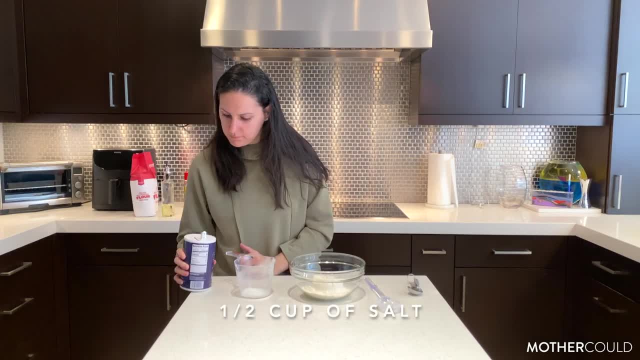 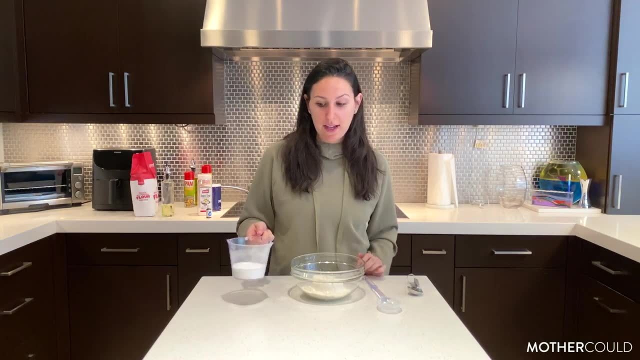 You don't have to compact the salt. You might be like whoa, that is a lot of salt, But the salt is what keeps it fresh on the shelf. So I would definitely go with the full half a cup of salt to make sure that it lasts your full six months. 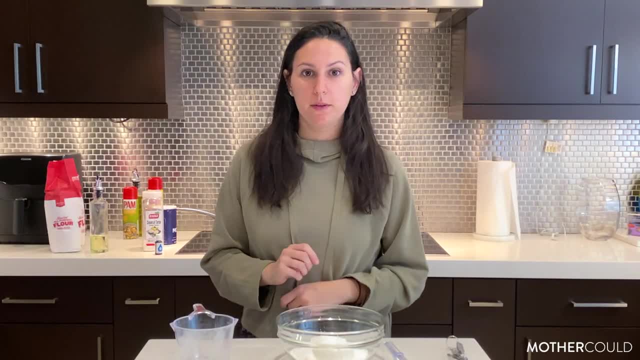 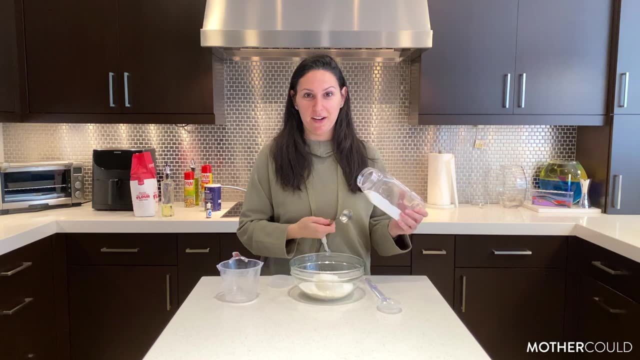 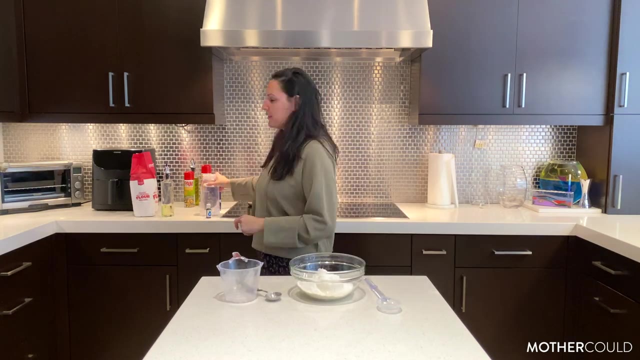 For my third dry ingredient, I'm going to add the cream of tartar. It's going to be two tablespoons of cream of tartar, Not exactly sure how to pronounce it, but you know what I mean. You could hear the water already boiling, so I'm going to leave it boiling because I want it to boil. 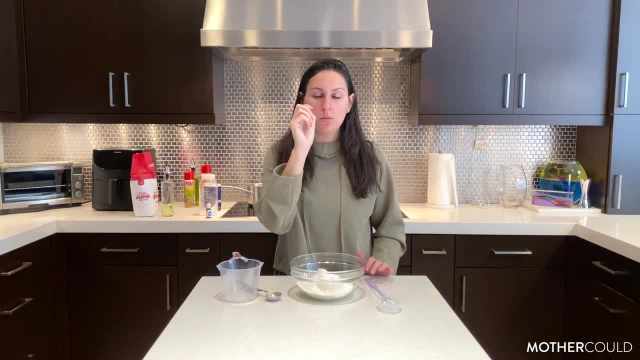 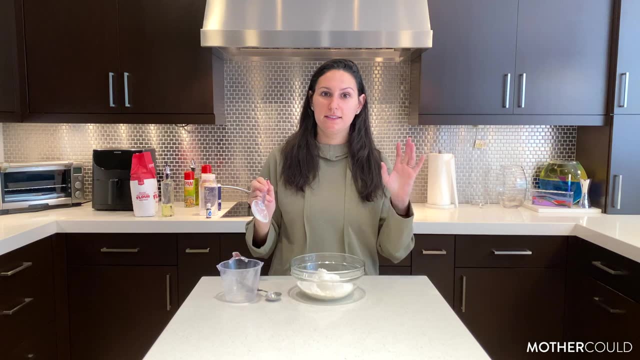 You can hear the water already boiling, So I'm going to leave it boiling, because I want it to boil, because i want it to be bubbling almost at the time that i'm going to pour it into here. it's exactly what's going to kill the bacteria in the flour, so it's important that it is boiling for now. 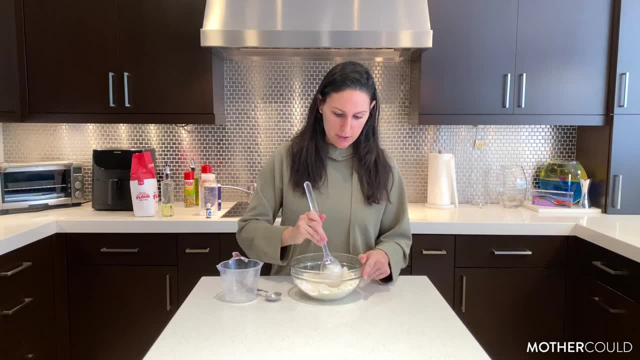 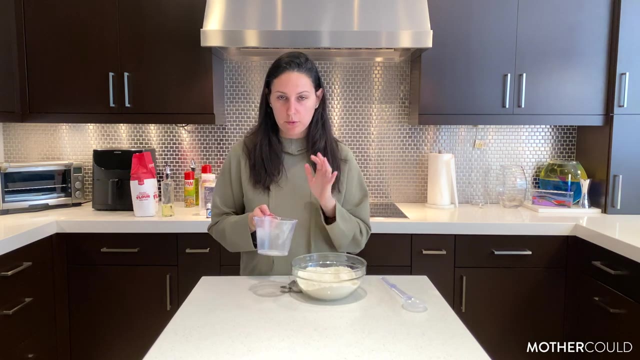 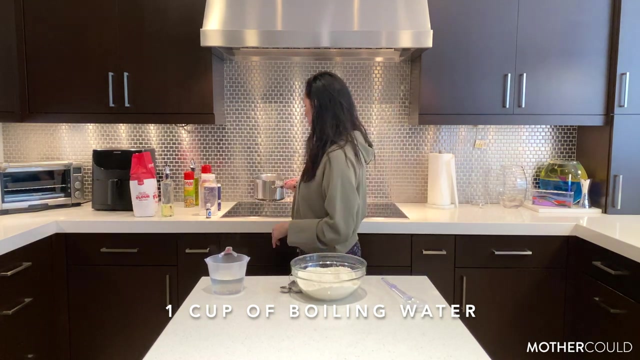 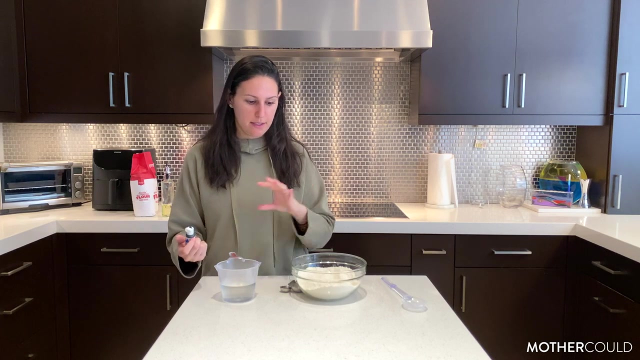 i'm going to mix all the dry ingredients together and make sure that they are very well mixed. so that's mixed, and i'm going to use again the same measuring cup to pour my water in, to add my food coloring straight into the boiling water. it helps with mixing the color evenly in the play-doh. 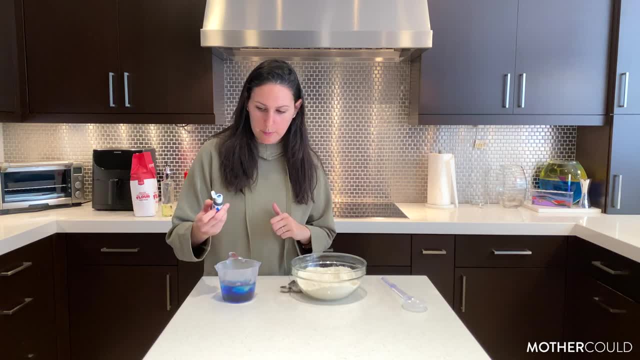 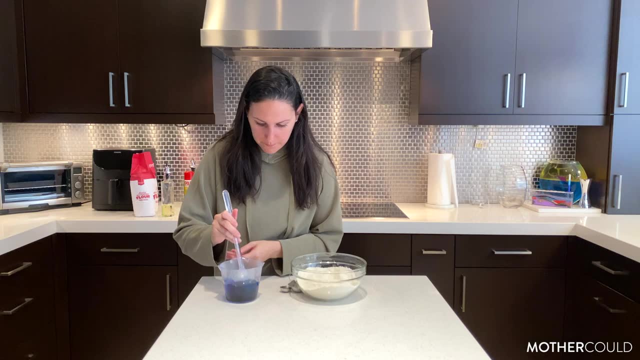 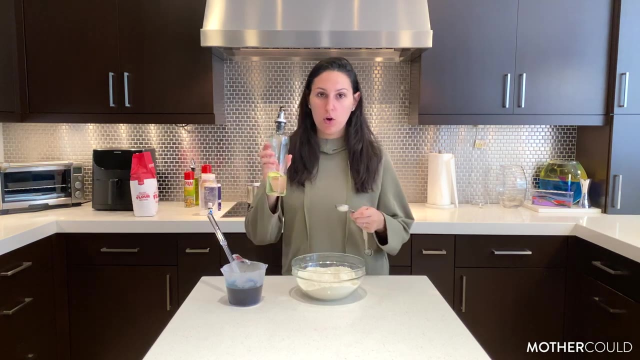 so i'm going to add about five drops of my absolute favorite food coloring. you know it's the Wilson color, right? um, and i'm gonna mix this up, leave it on the side for one second while i grab my oil and measure one tablespoon of regular oil. 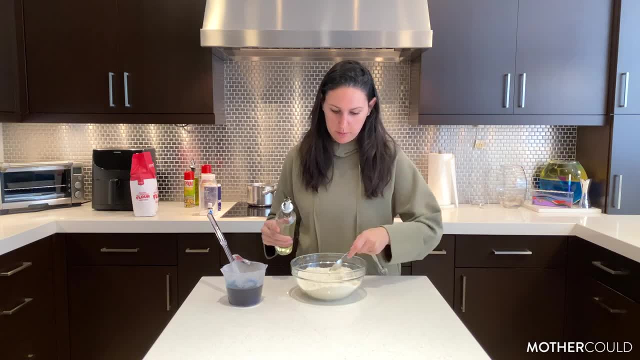 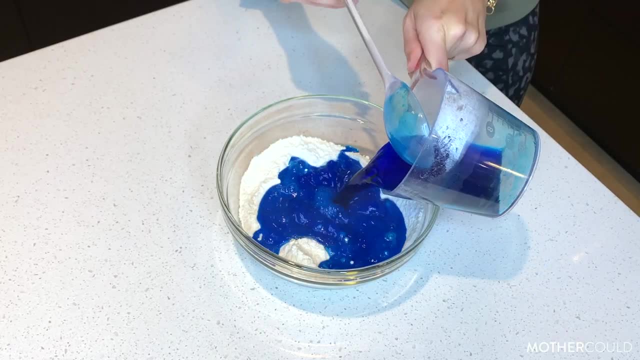 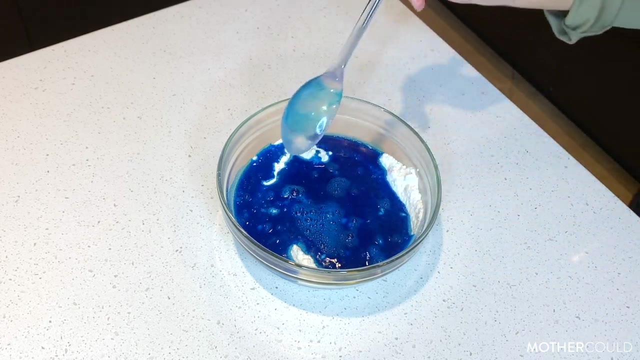 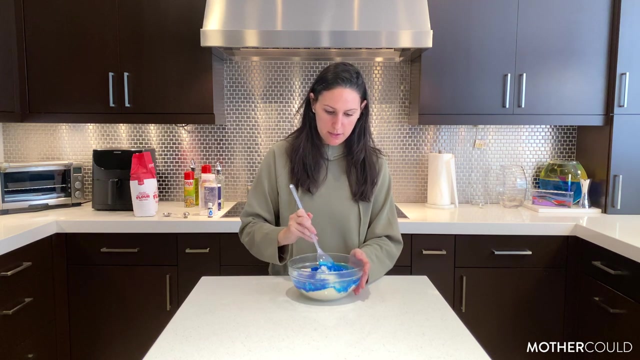 you could use any oil. i just go with the cheapest oil and quickly, quickly, pour in my boiling water. this is where you want to do this part as an adult- um, just so the kids don't get burnt- and you want to start mixing this immediately. like i said, the boiling water is what's going to kill the bacteria in the flour, so it's important. 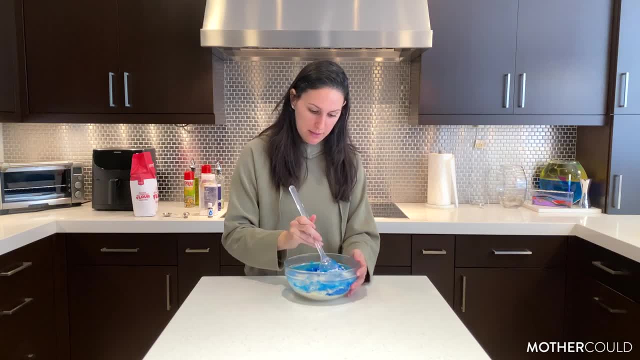 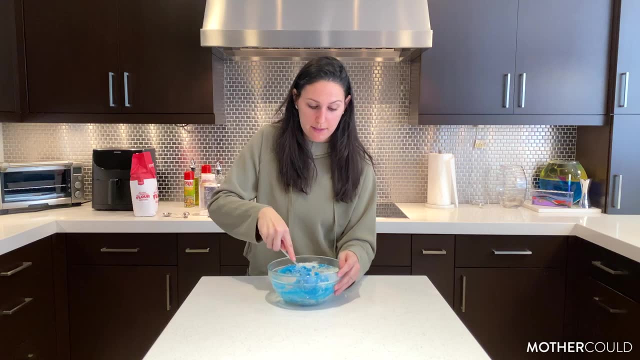 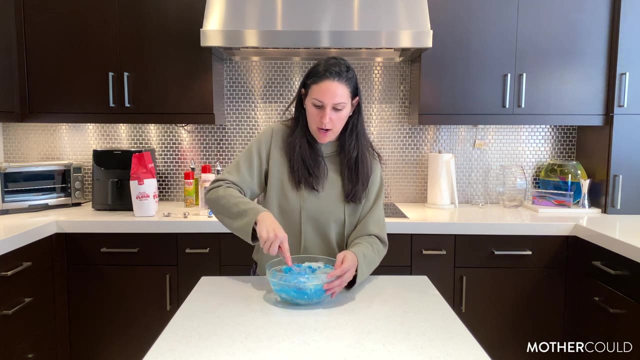 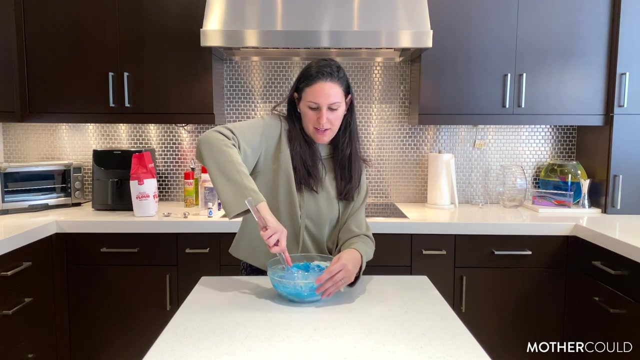 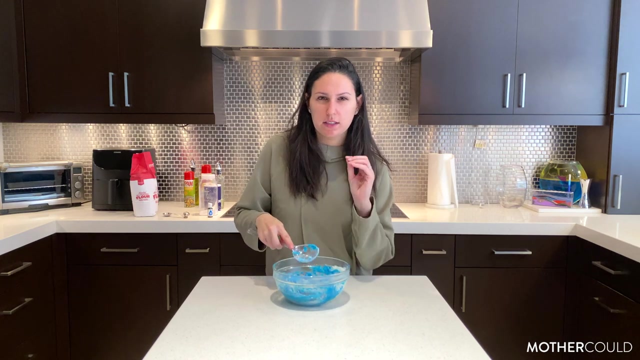 especially if you want the recipe to be taste safe. you want to keep mixing until it is cool enough that the oil is all mixed in to touch it. So right now it's still too hot in the boiling water. I'm just going to keep mixing in the flour with the dough and you can already see in the bowl how nice of a texture it is. Once you start to play with it with your hands, it really comes together. You don't feel the full consistency until it is completely cool. So if you feel like it's still a little wet and soft, that's because it has to cool down. 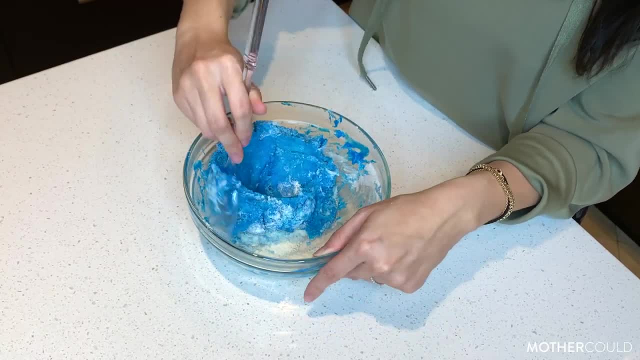 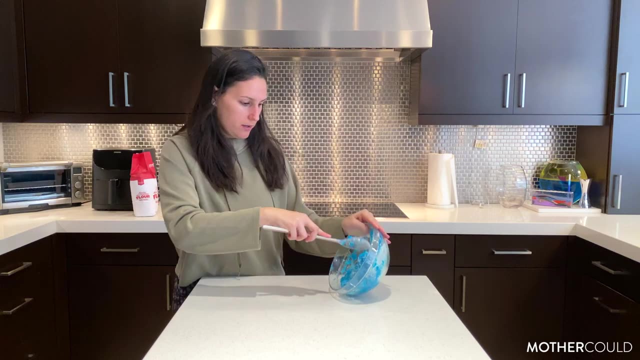 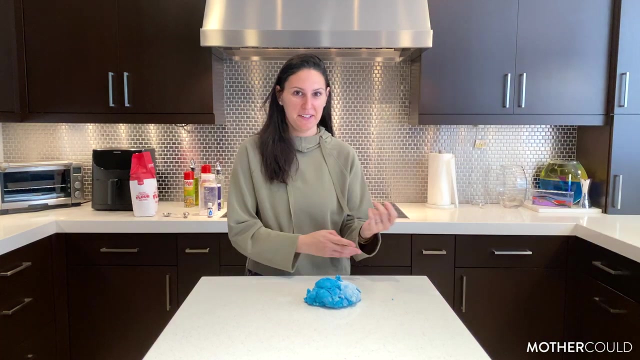 So don't add more water or more flour until it has been completely cooled down. Okay, so now I'm going to take it and I'm going to put it onto my table, Roll your sleeves up and start to play with it. So it's just cool enough for me. 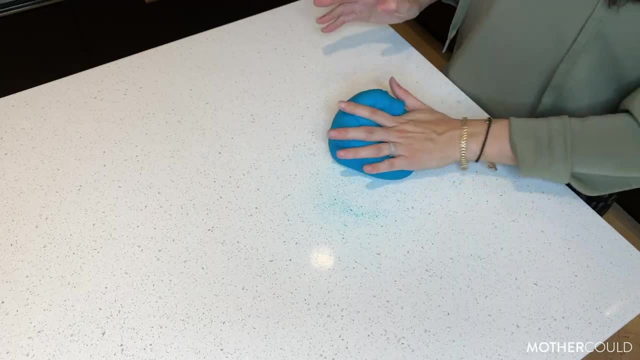 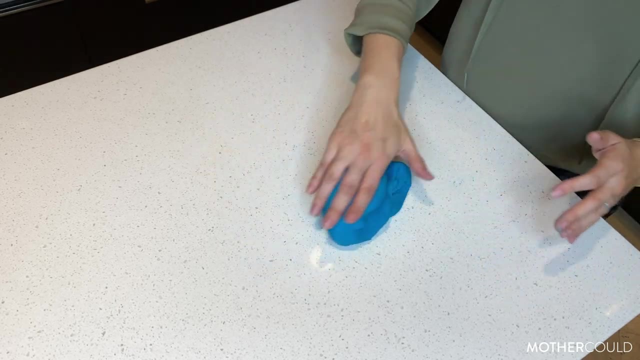 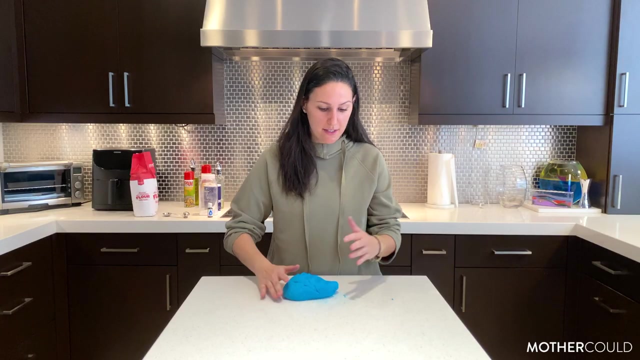 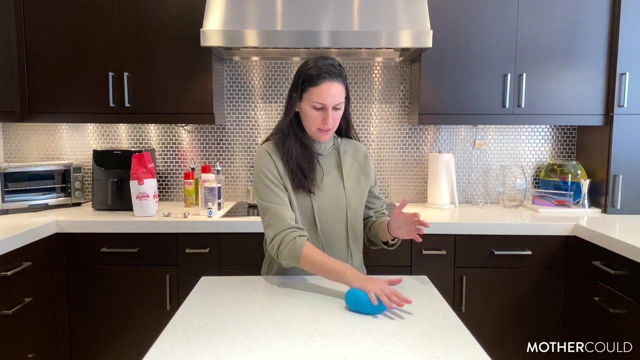 to touch with my hands already. It's already such a beautiful texture. Seriously, this is my absolute favorite Play-Doh, just because, as you saw, it came together really, really fast and it's almost like fail-proof. It also lasts six months plus on the shelf without any like special instructions or anything. It just is amazing. and the texture. 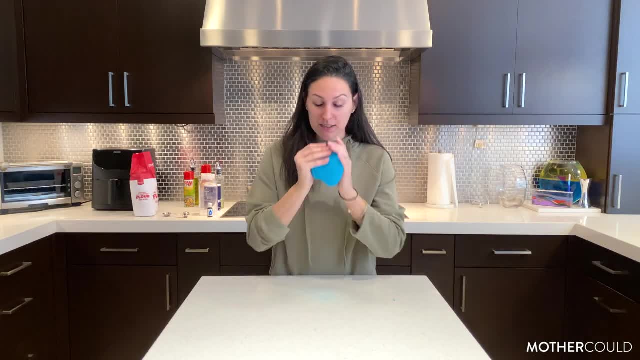 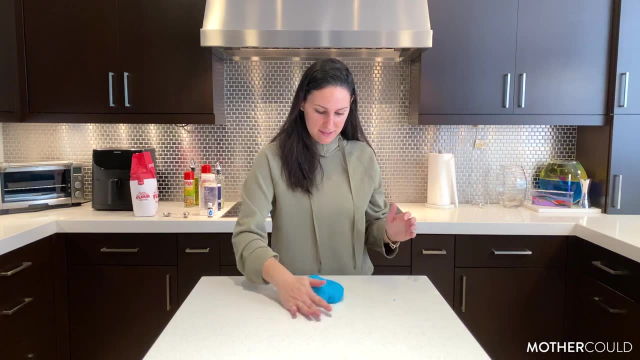 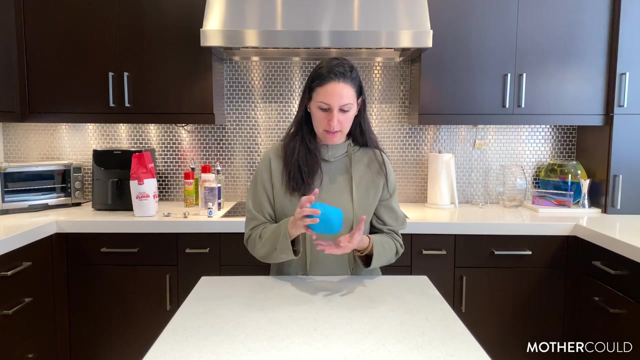 feels just like Play-Doh, It almost smells just like Play-Doh and it tastes just like Play-Doh for kids. So, yeah, my absolute favorite. you guys, You can see how fast that came together. Okay, so color is perfectly. even It's an amazing way. I'm going to wait for it to cool down completely. 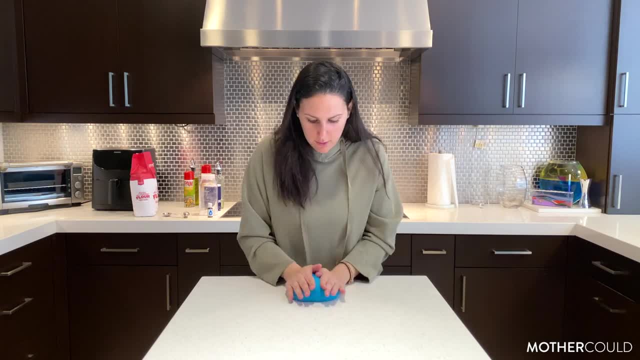 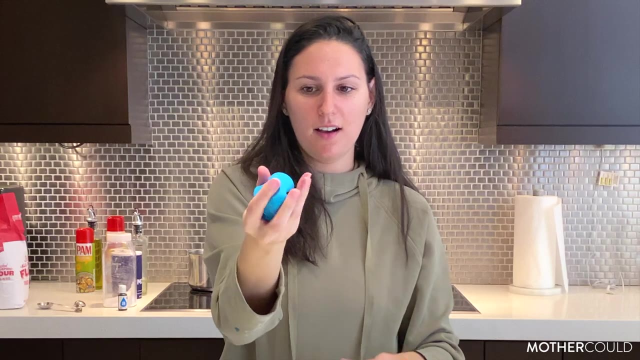 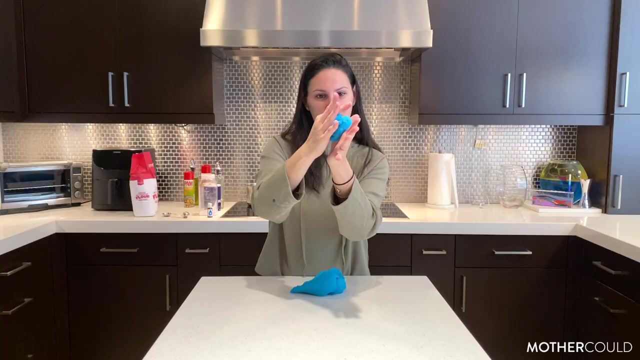 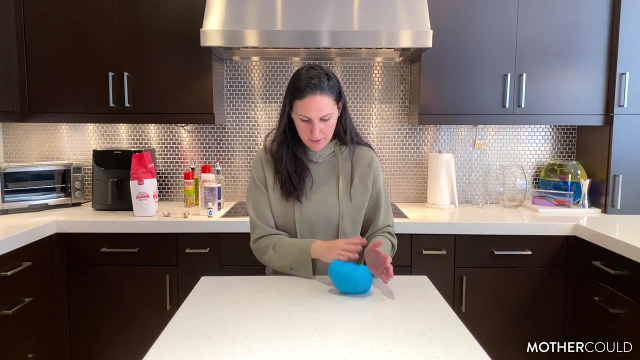 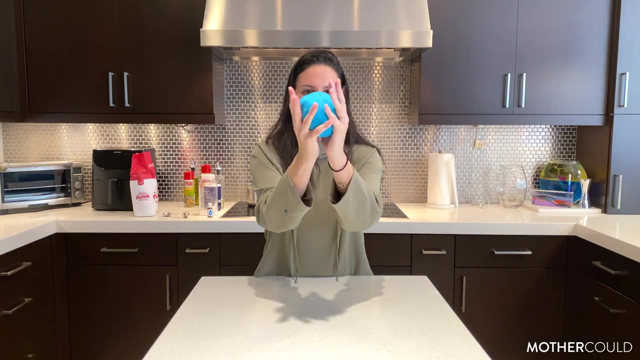 to get the true, true texture. but, as you can tell, my hands are not dirty at all, not sticky at all, Just amazing Shade and texture. Just like Play-Doh: Stretchy, soft, moldable, Amazing. And, as I do in all of my tutorials, make a nice ball and do the satisfying effect of ripping it apart. 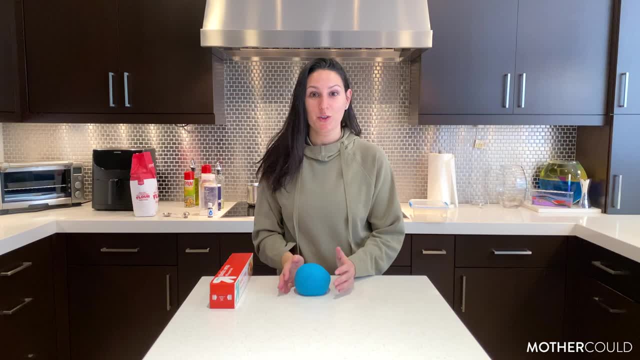 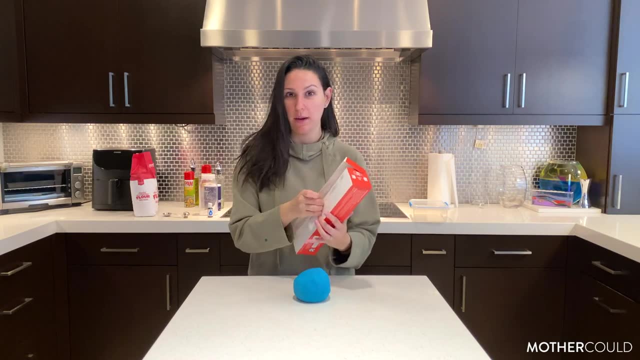 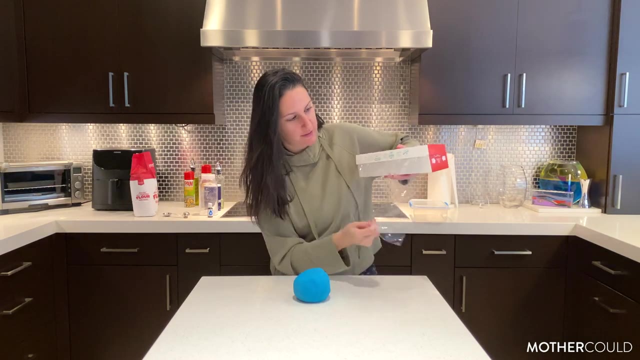 To store the Play-Doh. you're going to wait until it has completely cooled down and you're going to grab some plastic wrap, saran wrap, whatever you want to call it, And you're going to wrap your Play-Doh in it. So this is a little tricky, but this is how I like to do it.